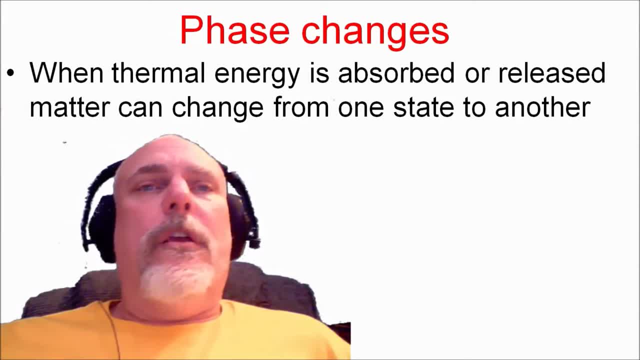 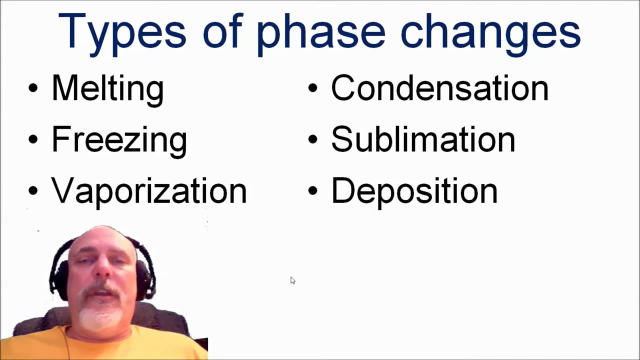 So energy needs to be absorbed or released for matter to change from one state to another. Like, for example, before we talked about melting, you need to add thermal energy to ice cream to get it to go from a solid to a liquid. The different phase changes that we are going to be studying in this unit are shown here on the screen. 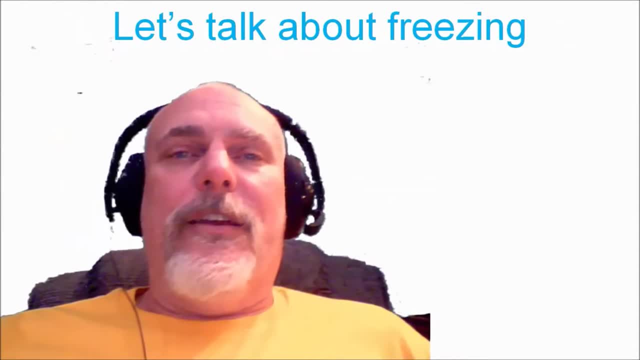 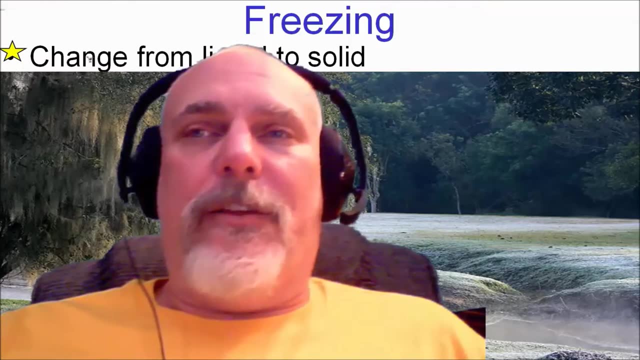 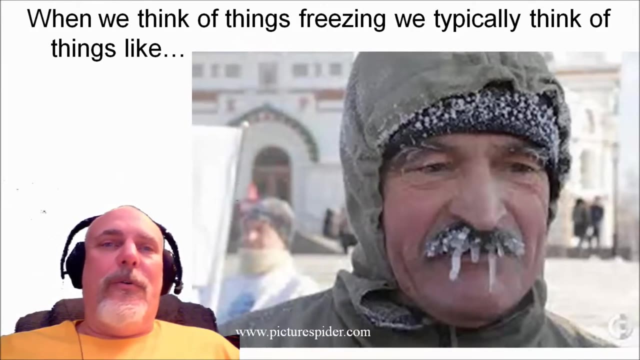 And, of course, like I just said, today's topic is freezing. Now let's talk about freezing. Freezing is defined as the change from a liquid to a solid. When we think about freezing, we typically think of things like Ice and snow and all kinds of very cold days and winter. 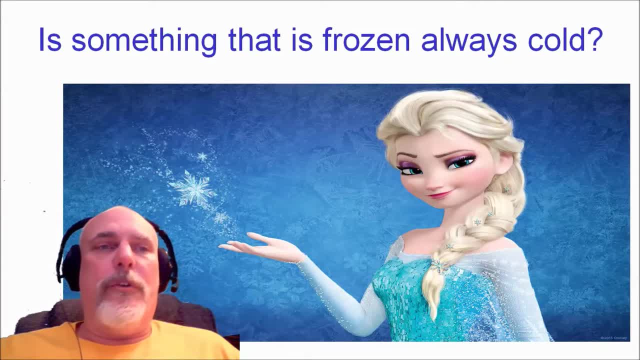 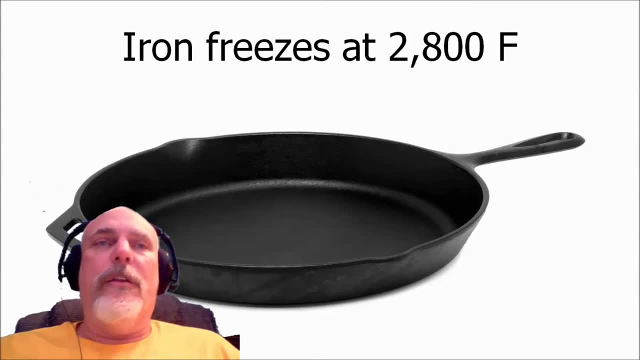 So is something that is frozen, always cold. Well, if you think about the definition, it's a change from a liquid to a solid. Well, if we have liquid molten iron, that will change to a solid at about 2,800 degrees Fahrenheit. 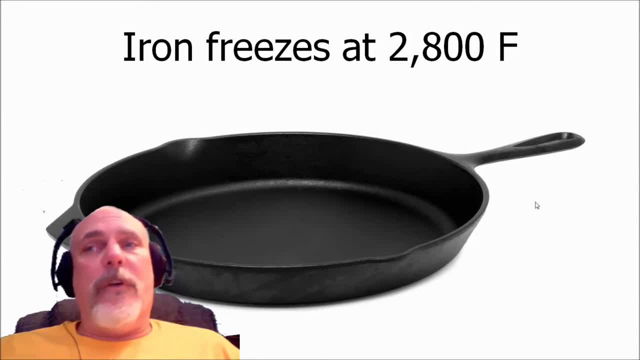 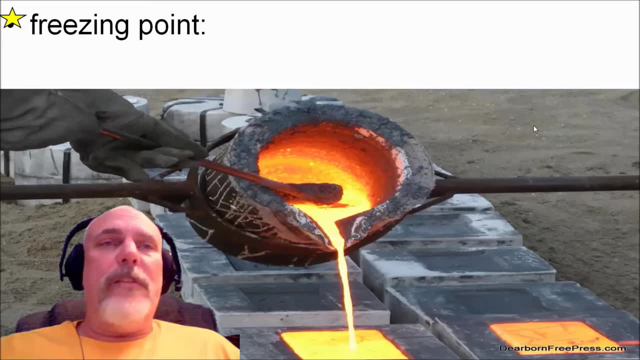 Most people would not consider that to be very cold. But again, when we're talking about temperatures, things are relative. object: It's frozen at 2,800 degrees Fahrenheit, So the freezing point is defined as the temperature at which a substance changes from a liquid to a solid. 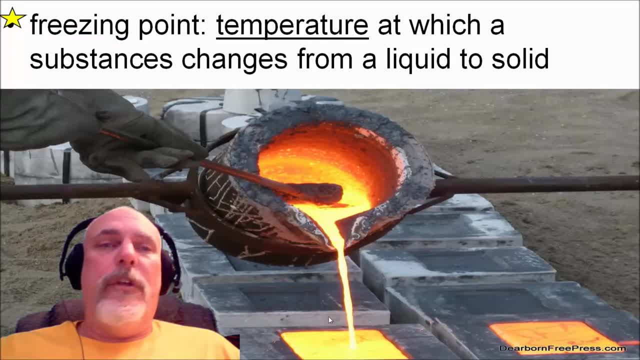 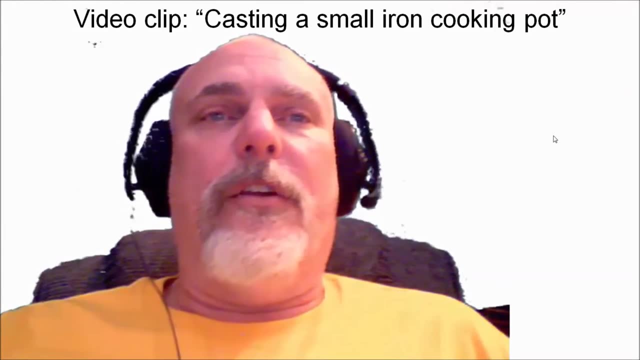 So here's molten iron, pouring it into a mold, And as soon as it starts dropping below 2,800 degrees Fahrenheit, it's going to start solidifying and forming solid iron. Here's a video clip Showing how to cast a small iron cooking pot. 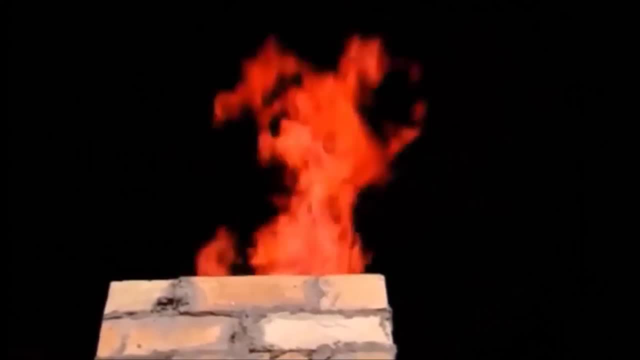 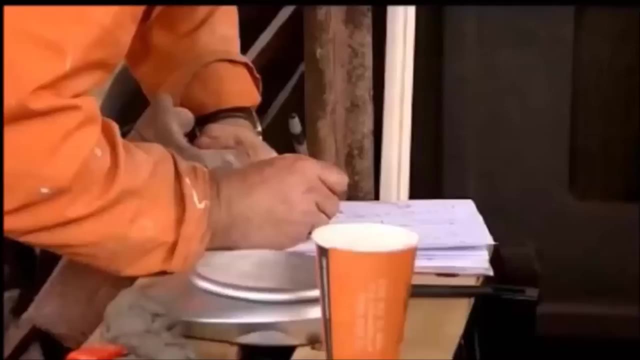 I think it's very interesting- closer to producing liquid metal. But for that liquid metal to be turned into a cooking pot, there's one last process they need to master with the help of self-taught expert Colin Peck. 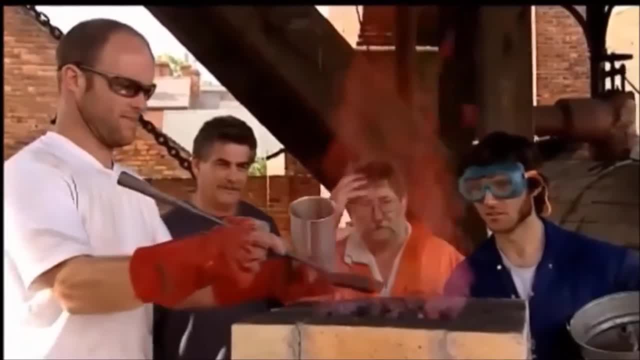 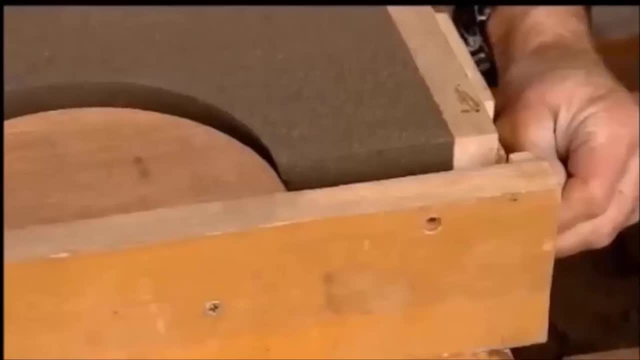 Hello Jerry, Nice to see you, mate. Green sand casting. Green sand means damp sand. When you compact it, you can form it into any shape you want. That's the inside of Guy and Maeve's boiling pot, For example. 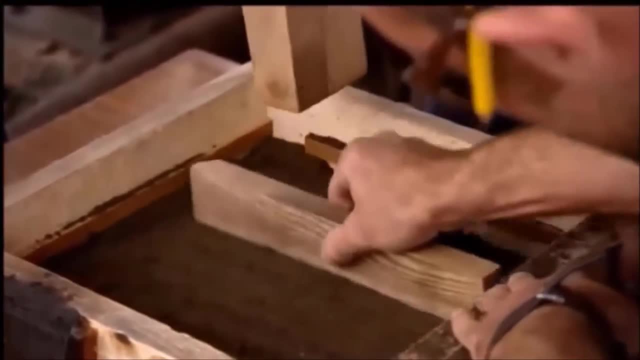 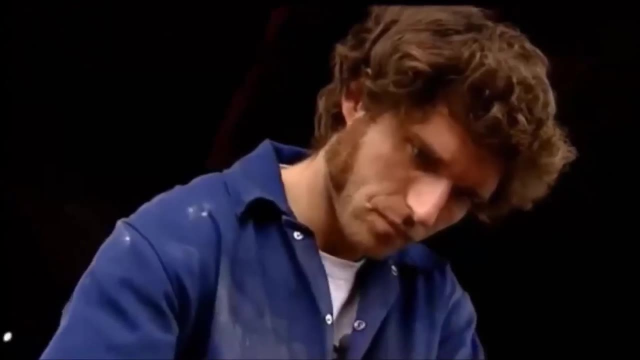 What have we got? A little bit firmer than that. Work your ways into your corners. Green sand casting was another British invention, patented by that man, Abraham Darby, at the start of the 1700s. Green sand was cheap and you could use it over and over again. 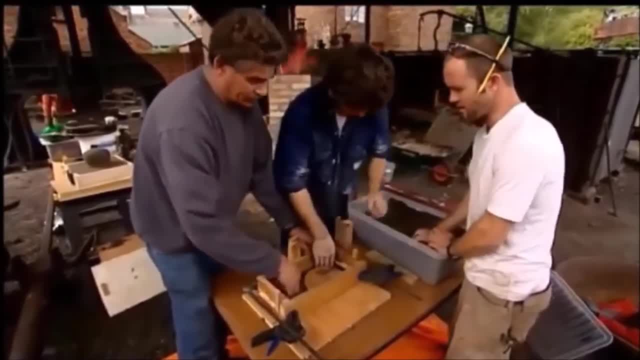 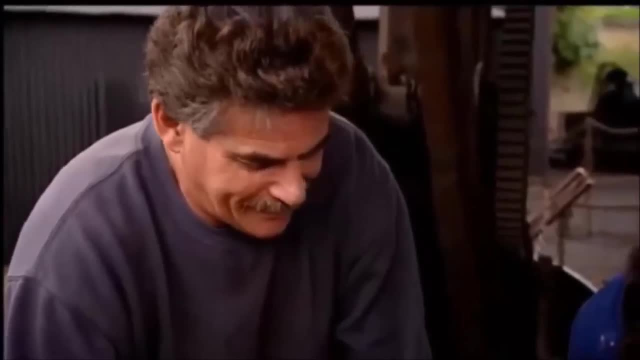 And with it large-scale production of cast iron objects like bridges, steam engines and even girders to build factories and aqueducts began. Give a little more effort than that. The boys make the green sand mold. They put the mold for their pot in four separate sections. 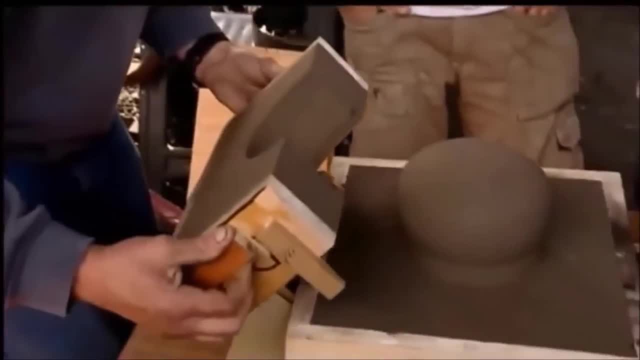 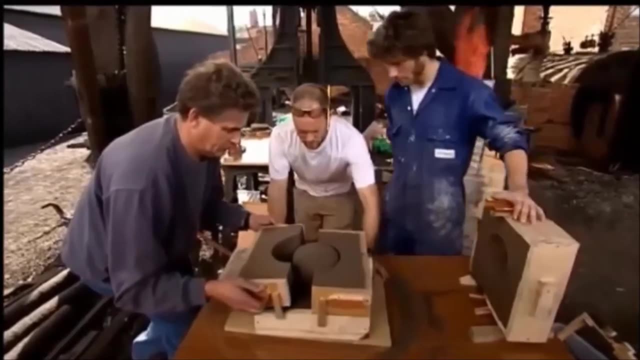 Okay, that'll do us nicely, But one slip, as they put the sections together and the mold will be wrecked. Once the parts are all joined, they leave a pot-shaped gap between them, into which the boys will hopefully pour their molten iron. 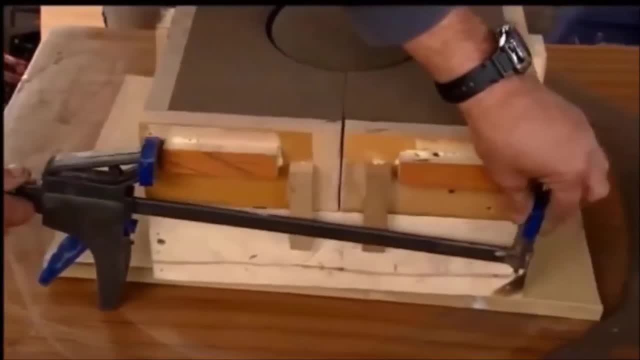 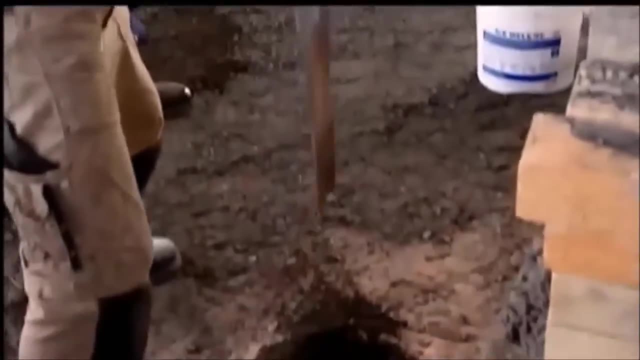 Well done you, But it won't be until they break the mold apart at the end that they'll discover if what they've made is good enough. After days of work, it's time to break open the clay seal at the base of the furnace. 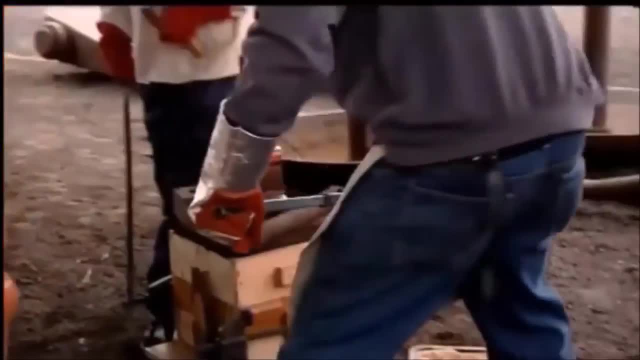 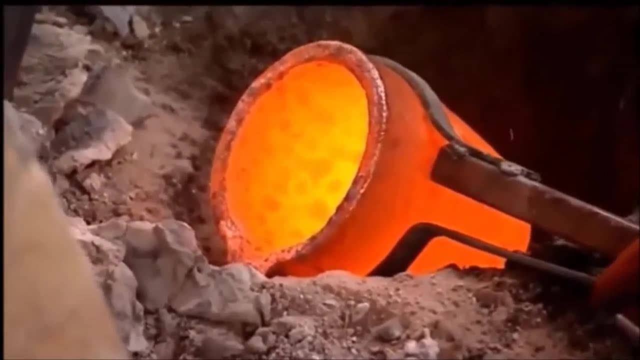 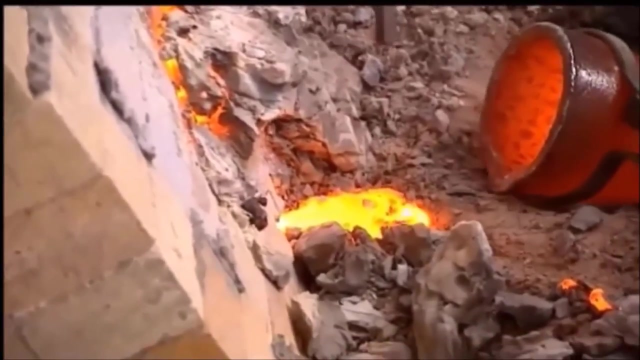 As Guy stands ready to release the liquid iron, Colin moves into place with a red-hot crucible, heated in his own mobile furnace, ready to catch the boys' precious metal. She's coming, she's coming Success. They've made molten iron. 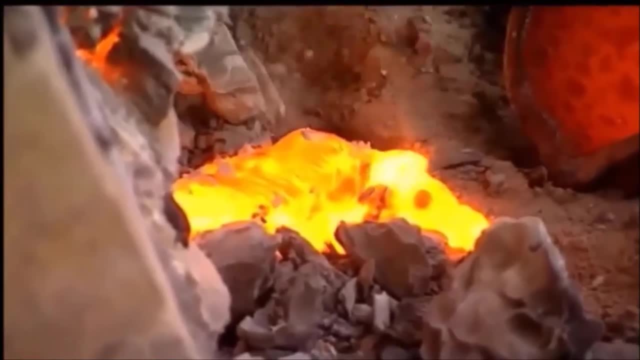 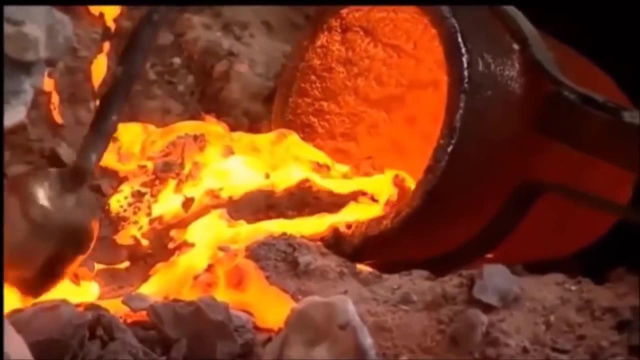 Or have they? It quickly becomes clear that there's a problem. The metal isn't liquid enough to flow properly, It's not hot enough And there's a doubt about how much is actually metal and how much is just the molten impurities called slag. 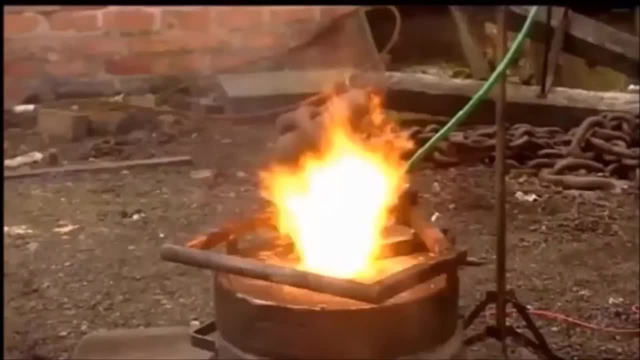 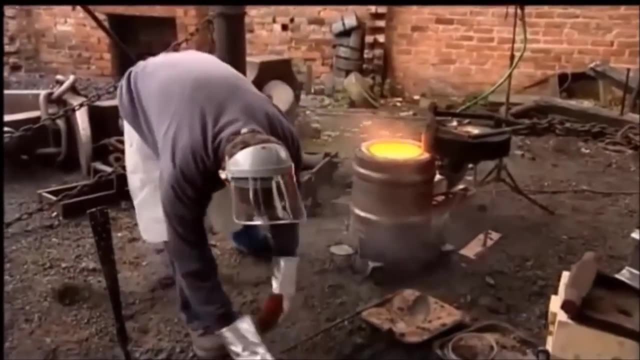 It's time to act fast. Colin reheats the mix in his portable furnace and adds a healthy dose of scrap metal to make absolutely sure there's enough molten iron produced to fill the mold. It's getting close to temperature here now, so I'm going to need the mold down there. 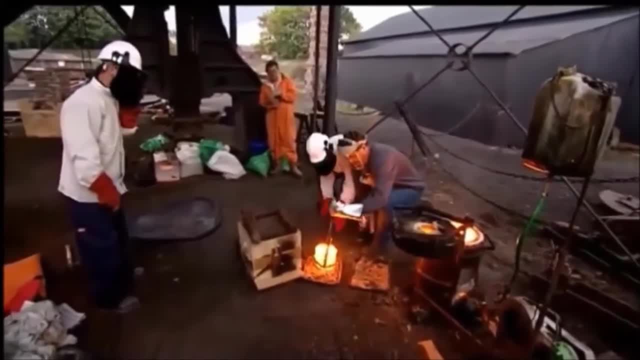 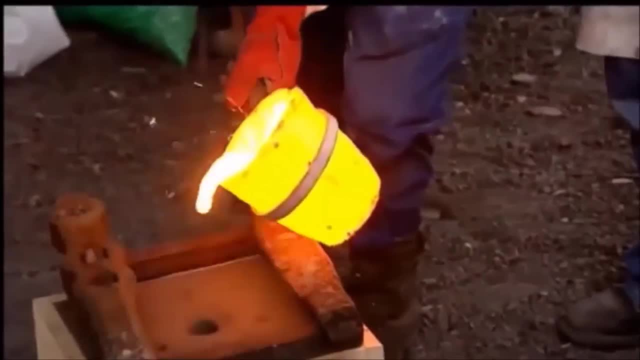 Finally, Colin lifts the iron from his furnace and, having scooped off the slag that's risen to the surface, it's over to Guy. Right, pour away, Get in that hole. Other floor, You've got to go out of the spout, Guy. 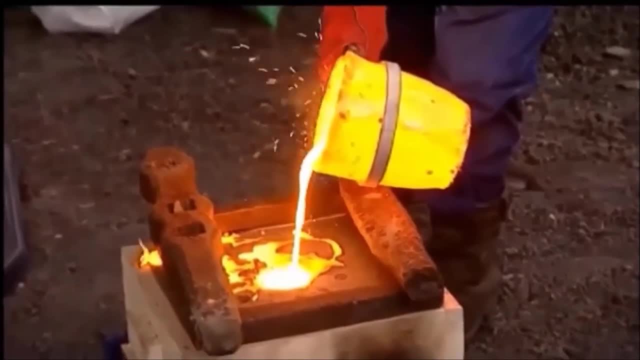 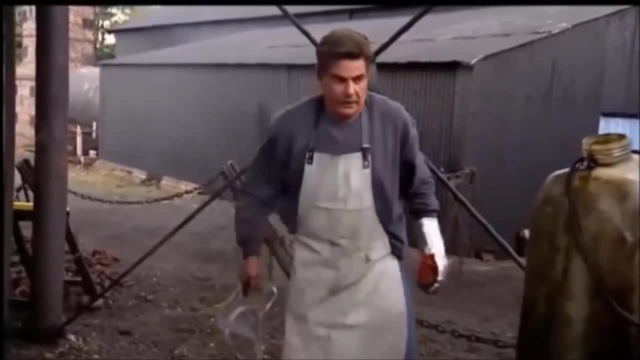 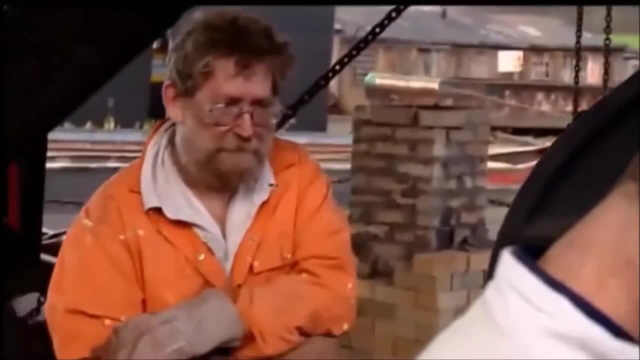 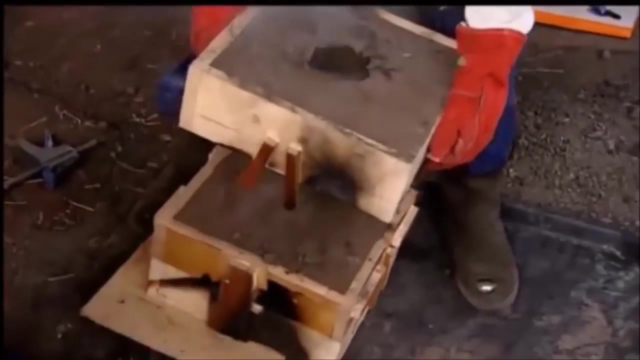 You could have just let it come outside. All they can do is wait for the metal to cool to see if disturbing the securing weights has ruined the mold And whether Gerry's iron has done the job. If it hasn't, two days' graft will have been wasted. 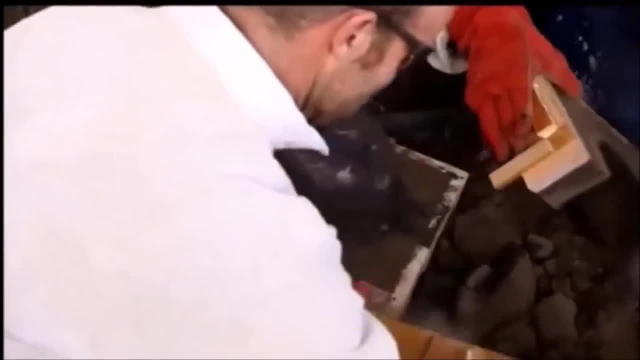 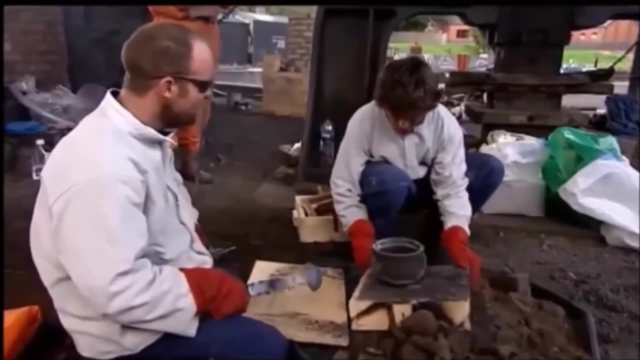 The sand is removed and success. Want to see your pot guys, There you go: A complete pot, It's all there. Woo-hoo. That's quite splendid, don't you reckon? Well done, Mark. Eh Can't do it without them, chaps. 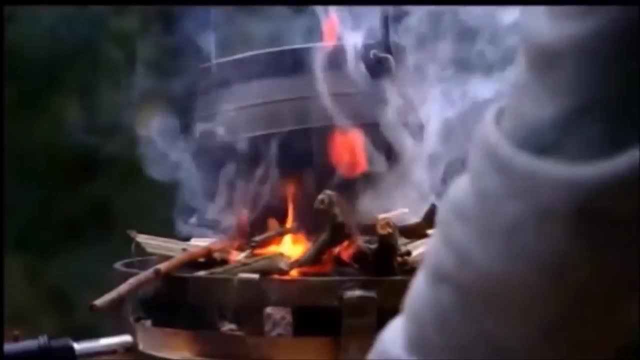 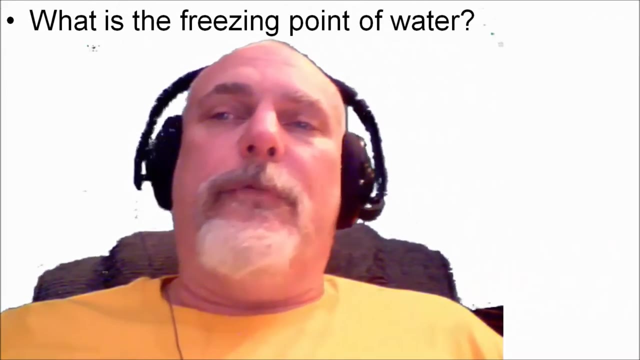 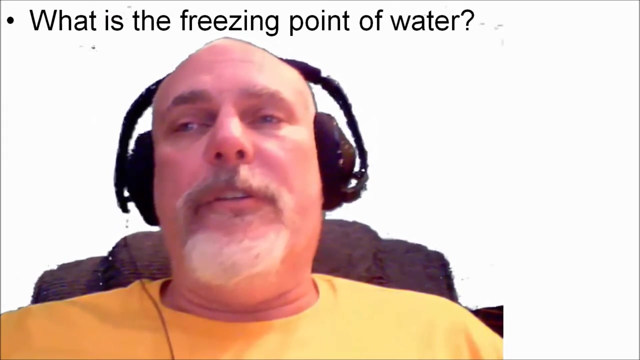 Right, We've earned ourselves a brew. I reckon Gasping Yeah. When we're talking about melting points and freezing points and phase changes, we often will be thinking about water. So what is the freezing point of water? And you've got to remember what freezing point is a temperature. 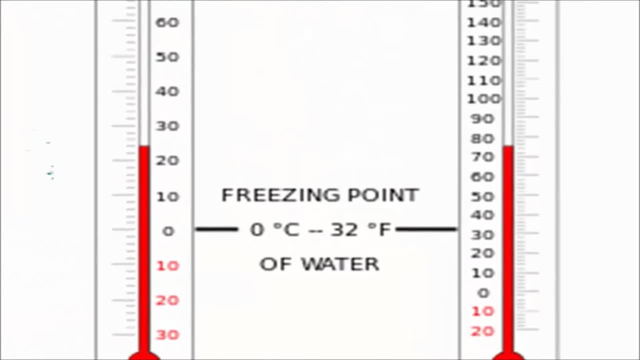 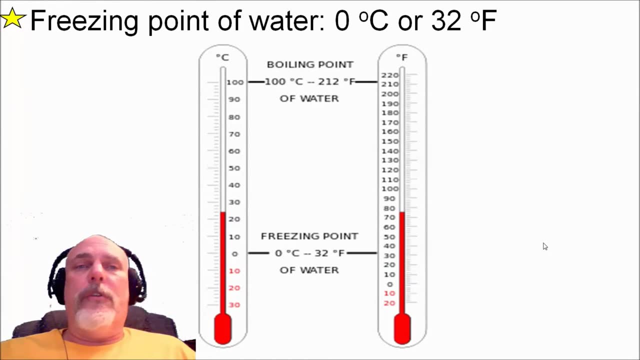 The freezing point of water is 0 degrees Celsius or 32 degrees Fahrenheit, They are both the same, Just like if you have 1 inch or 2.54 centimeters. they're the same length If you have 2.2046 pounds. 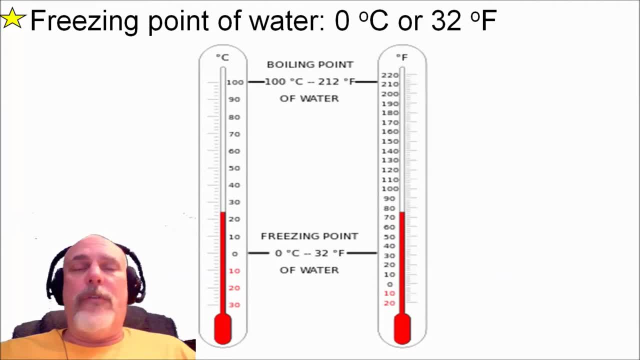 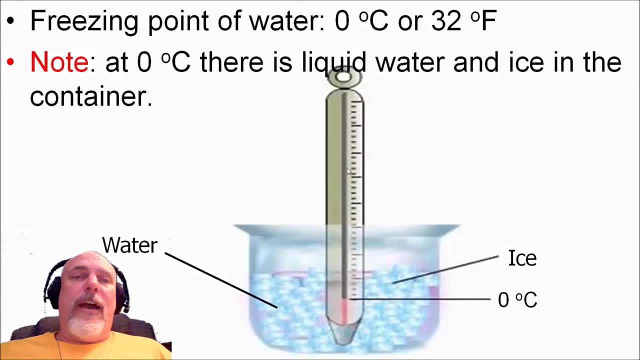 that's the same as 1 kilogram. Even though the numbers are different, it's the same measurement. Here's a thermometer stuck in an ice water bath. The thermometer reads 0 degrees Celsius, But please note that there is liquid water and ice. 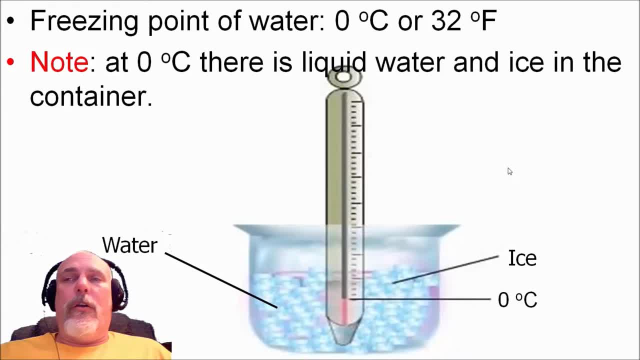 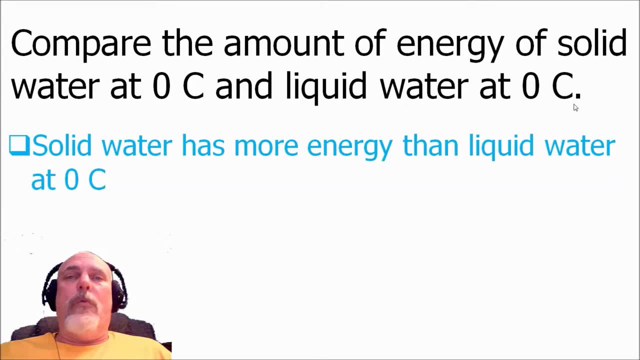 solid water in the container, even though they are both at 0 degrees Celsius. Let's compare the amount of energy of solid water at 0 degrees Celsius and liquid water at 0 degrees Celsius. Which one of these, which one of these choices, is most correct? 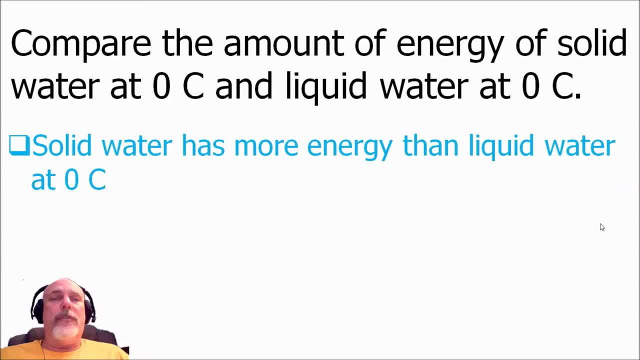 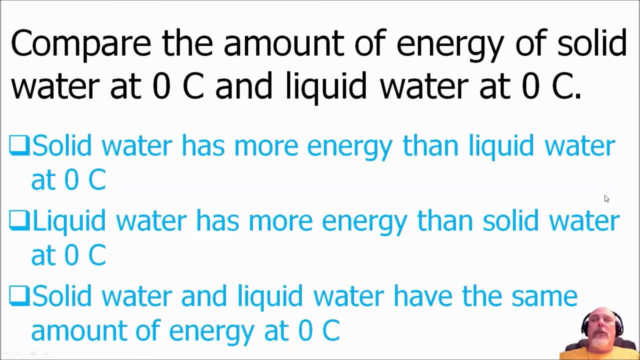 Is solid water has more energy than liquid water at 0 degrees Celsius. Liquid water has more energy than solid water at 0 degrees Celsius. Or is it solid water and liquid water have the same amount of energy at 0 degrees Celsius? What do you think? 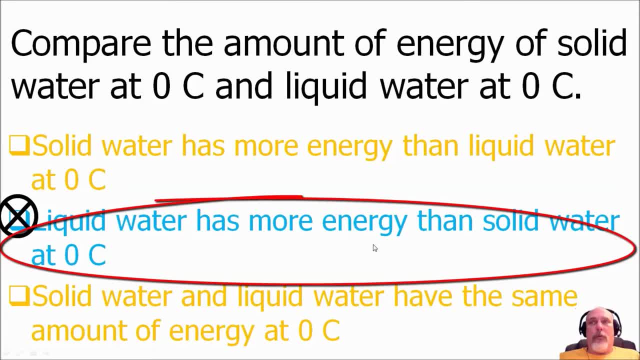 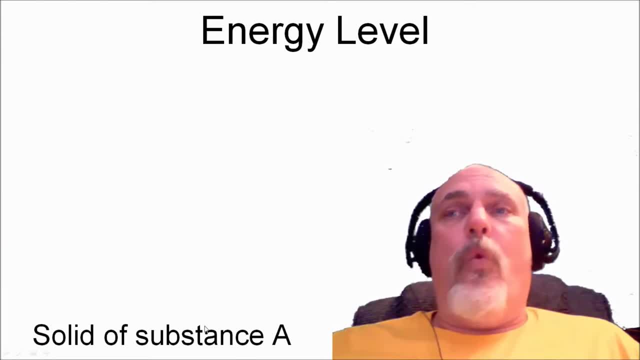 Well, hopefully you chose the middle one. Liquid water has more energy than solid water at 0 degrees Celsius. Well, we've talked about energy level. The energy level of a solid substance like water- so that would be ice- is at a lower energy level than the liquid of that same substance, like liquid water.